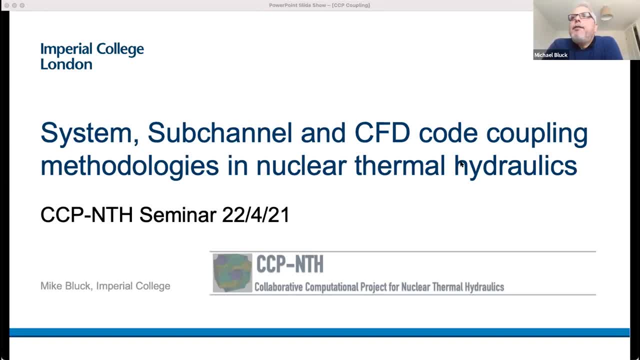 Yes, So I wanted to give an overview really of the work we do at Imperial in coupling particularly, obviously, systems codes, which we mentioned, but sub-channel codes and CFD. I won't be going into sort of great detail in any one particular area, but to give you an idea of some of the challenges we've met. 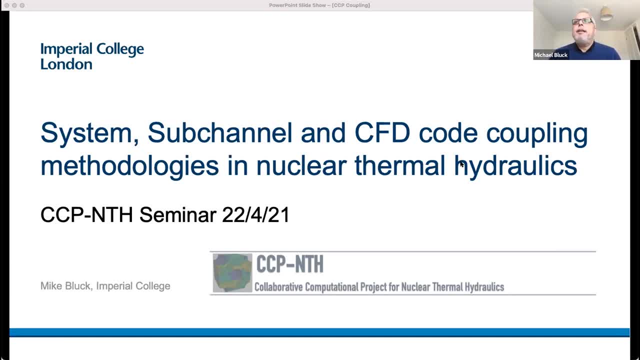 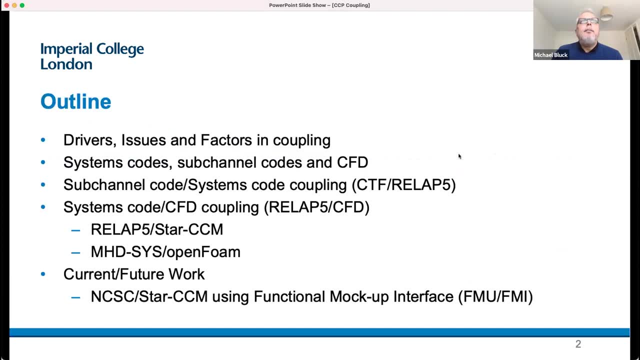 Not all of which are particularly technical, it should be said. I think that's something that has to be borne in mind, So let me- Sorry So- just a brief outline. I'll mention the drivers issues and factors in coupling. 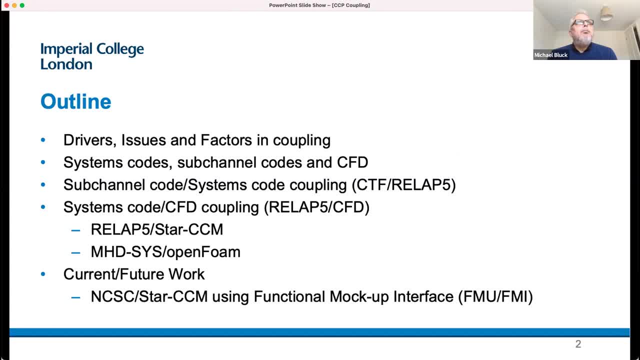 As I said, these aren't always technical And I'll just mention sort of the bits about the various codes that we're talking about or the types of codes more specifically, And then I'll give The body of this will be about some of the experiences we've had in code coupling in various forms, whether that's CFD and systems codes or sub-channel codes and systems codes, and in various forms one way or another, over a sort of period of a decade really. 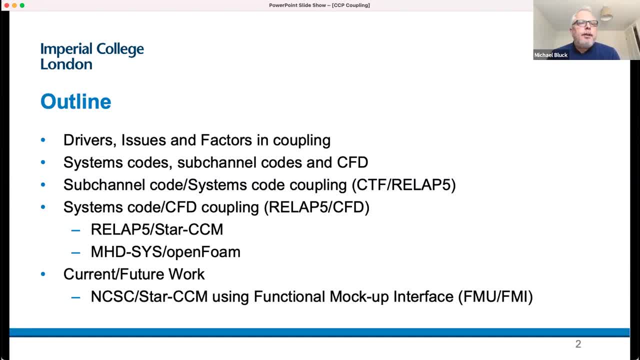 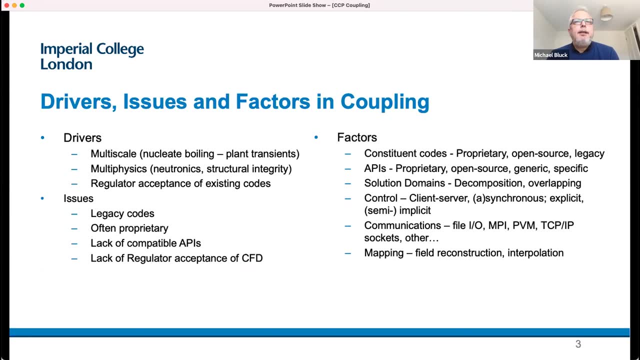 So You know, this particular set of seminars is very interesting. It's interesting to see how far things have come and, in some ways, how far things haven't. So, first of all, some of the drivers. So clearly, the need to model multi-scale phenomena, from nuclear boiling all the way up to full plant transients, is the main driver. 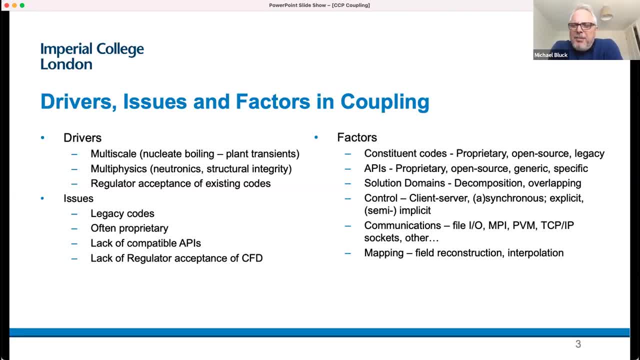 There's multi-physics, which has been mentioned. I won't be really talking Particularly about that, although there's a multi-physics element a bit later on in a particular implementation. Another driver is there's broad acceptance of lots of existing codes in nuclear. 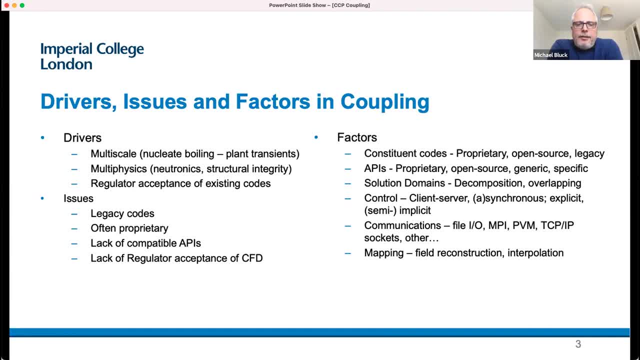 There aren't very many And the regulator feels comfortable about these And, as I think Antoine said earlier, that seems to be a good starting point. Nevertheless, it doesn't obviate the need to do lots of validation of what you get. 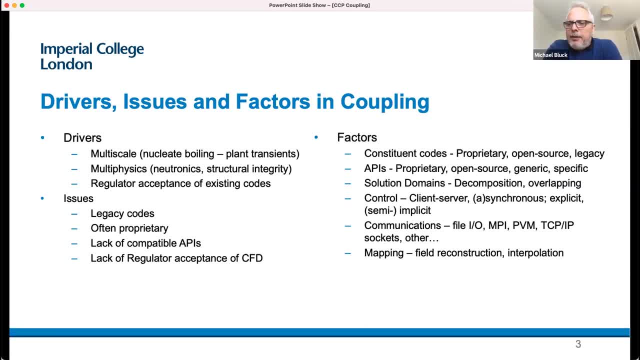 So the issues broadly. there's a lot of legacy codes And when you're talking about the recent developments, the important nature of legacy codes is often forgotten. They're often proprietary. So the sort of what are quite straightforward adaptations needed scientifically, mathematically, computationally, are very difficult to do in practice. 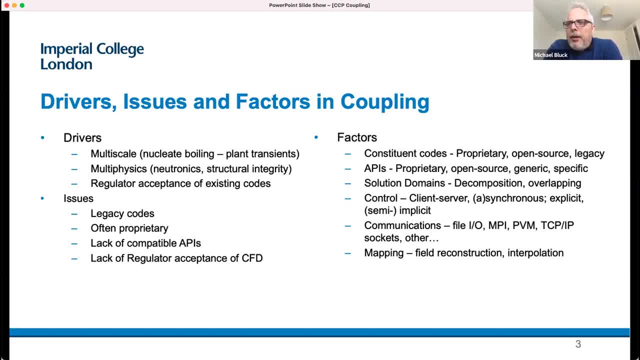 Lack of compatible APIs. You could fill a Scrabble board with the various APIs and protocols that are available And this kind of thing. Yeah, In that context there's also a lack of regulator acceptance of CFD, at least in the UK. 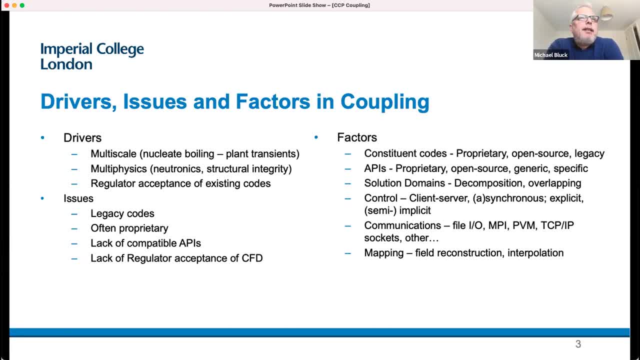 So the need to couple to CFD is clear. Actually getting the regulator to accept it is another issue. So collectively there's a strong driver to develop code coupling on a number of issues, And so that leads really in a sense. what follows is really a discussion of the sort of factors that influence code coupling. 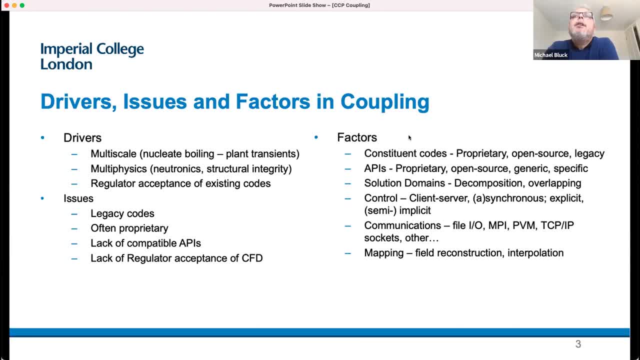 So, firstly, primarily, you've got the constituent codes. They could be proprietary, They could be open source, They could be legacy. In addition to that, there may be accessibility issues, APIs, the application programmer interfaces. again, these could be proprietary. 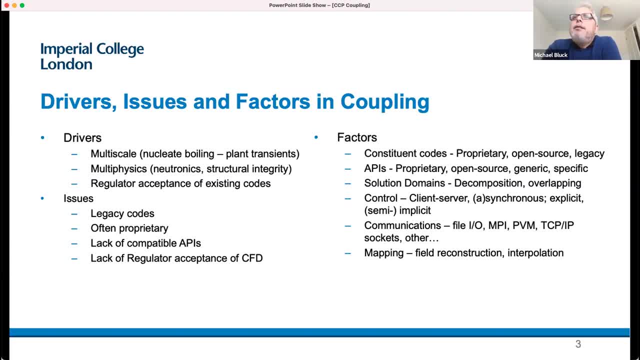 They could be open source, generic, specific or nonexistent at all. Then you've got solution, domain choices And, as Antoine pointed out earlier, there's domain decomposition or domain overlapping. I'll be concentrating on domain decomposition as a counterpoint to Antoine's overlapping description. 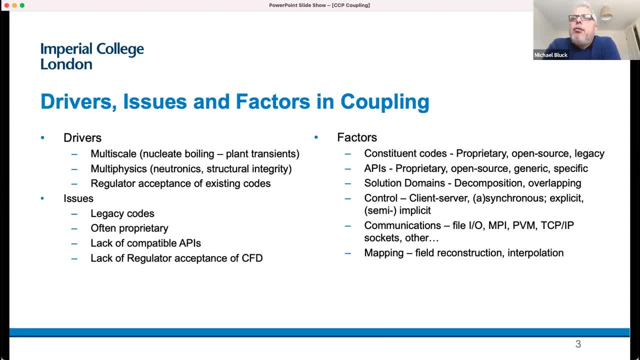 And then there's all the matter of control. Is it a client-server model? Is it asynchronous or synchronous? On the numeric side, is it an explicit algorithm or implicit or semi-implicit? So that's a sort of control issue. And then you've got communications. 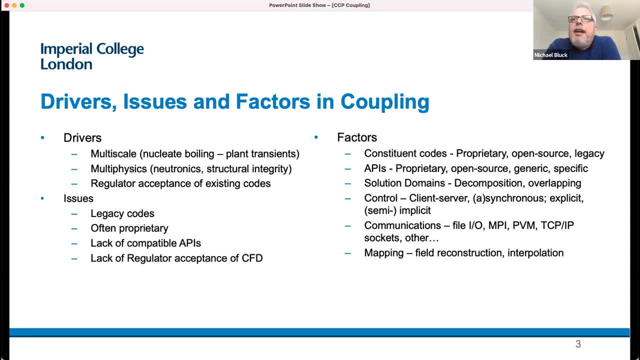 You know anything from- and no, it's not dead yet- file IO, sort of transfer of information by file IO, messaging paradigms like MPI or PVM, right down to TCPIP socket calls, And then, of course, embodying those are lots of protocols that embody these in one way, shape or form. 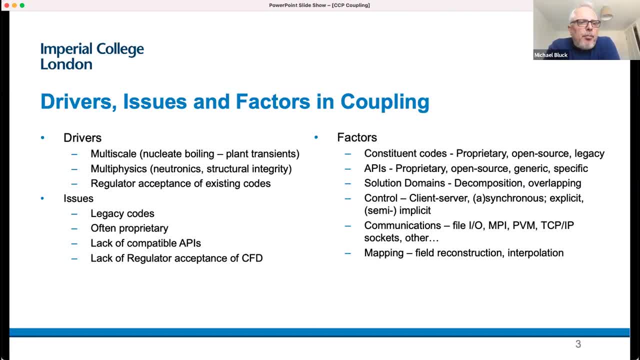 And the final one- it's not an exhaustive list- is the mapping between them: Field reconstruction, so profile reconstruction, you know, mapping from a systems code to CFD and so on, And any interpolation of. you know different codes are often dealing with different quantities. 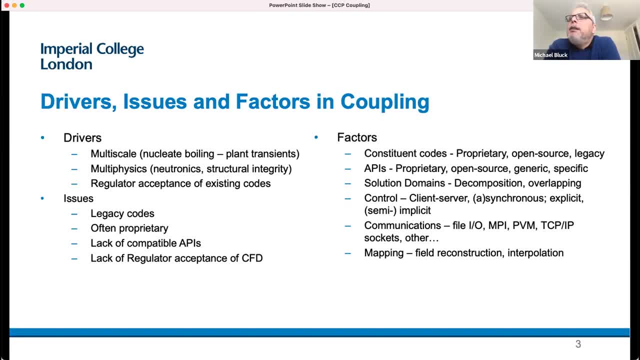 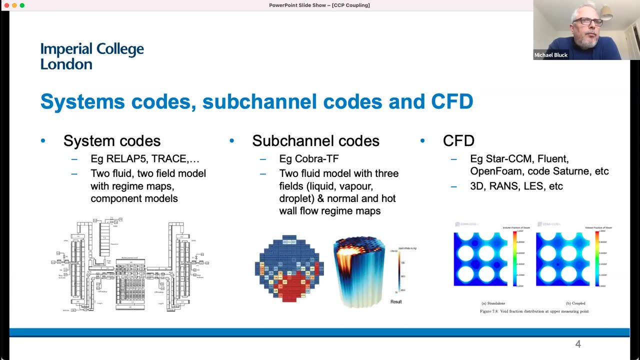 And they're not necessarily in the same place And they're not necessarily interpolated or treated in the same way. So these are the sorts of factors- And I'll mention these factors in each of the sort of cases I'll be looking at. So we're covering sort of three broad areas really that encompass broadly the way we treat thermal hydraulics. 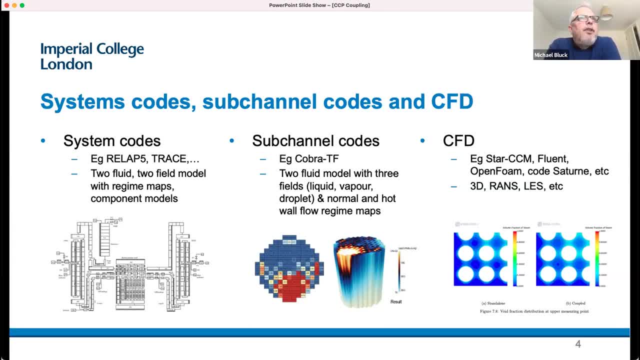 On the left we've got systems codes, We have five trace guitar et cetera. So we have five examples, two fluid, two field model. It has sort of embodied in there lots of regime maps, flow regime maps, correlations, sort of whole component models. 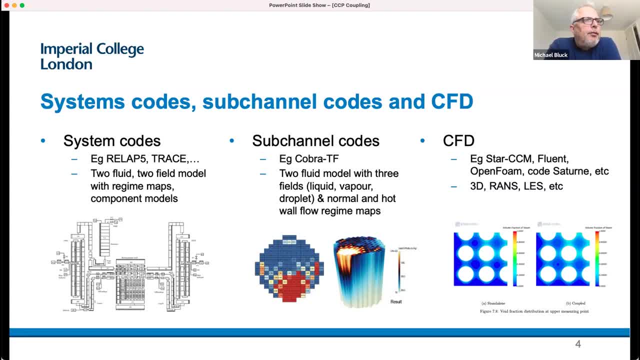 And underlying. that is essentially a one-dimensional description of the flow, Although there are 3D- Relapify 3D being an example- but they're not heavily used And then they are quite limited. So you know, systems code is fine for much of the plant, depending on the degree of detail you require. 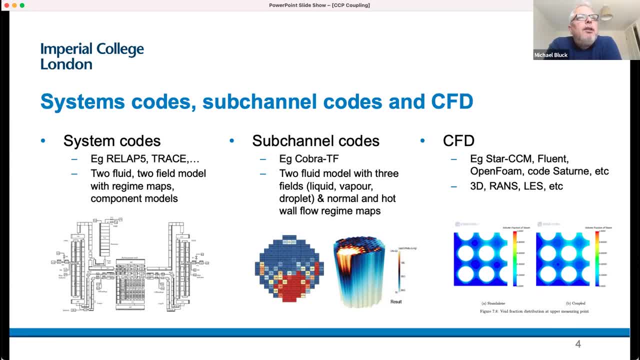 But in the core. it's pretty woeful Describing the core as three pipes or even less. You know, if you need more detail in the core, you look at it. If you need more detail in the core, you look at sub-channel codes. 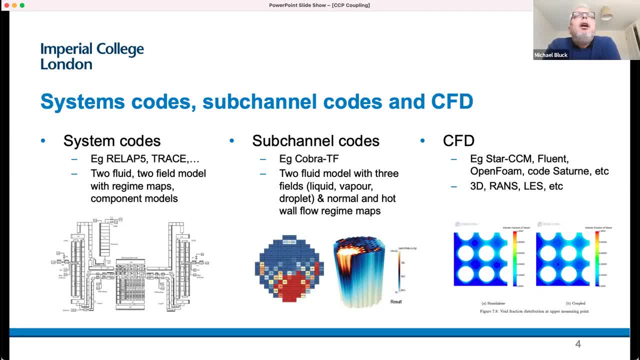 For instance, Cobra, Cobra TF and so on, And these are sort of more evolved models again, but similarly simplified models of the flow, But they incorporate more detailed models of, in the case of Cobra, all of liquid, vapor and droplet flow regimes. 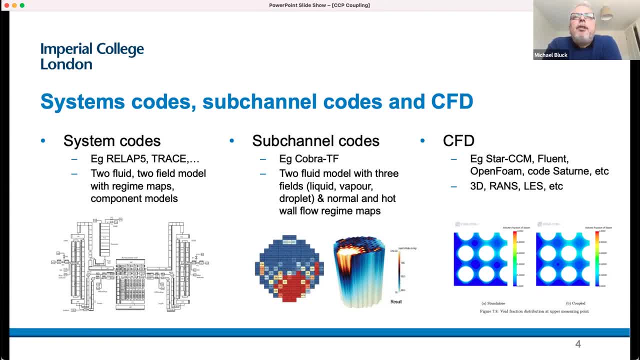 And additional models to take into account Particular nature of the core. And then, on the right, we've got some of the higher fidelity models, Lots of commercial codes, Some open source, open foam codes, etc. Embodying the capability to do 3D, RANS, LES, even down to DNS. 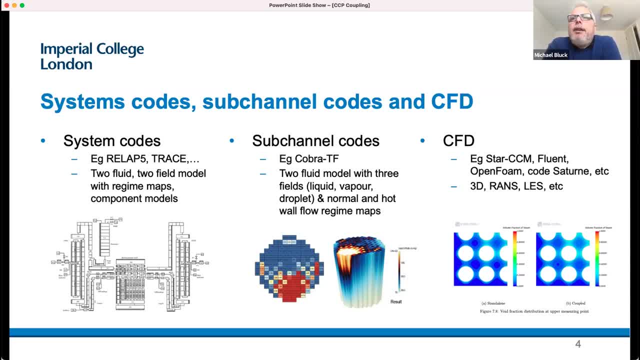 And so you know these are important where we really care about the flow detail, And that can be anything from a T-junction, if you like, or flow within sort of two bundles during transience, as you might see below. So there's a clear sort of range of scales there. 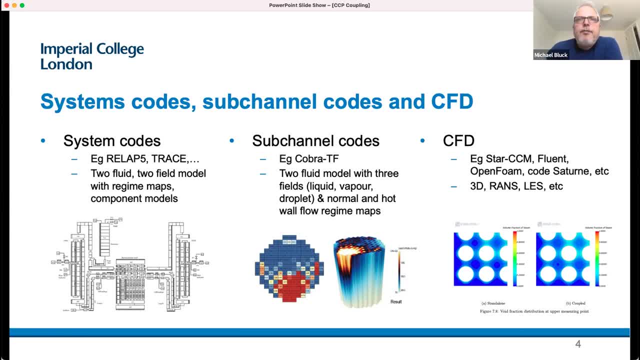 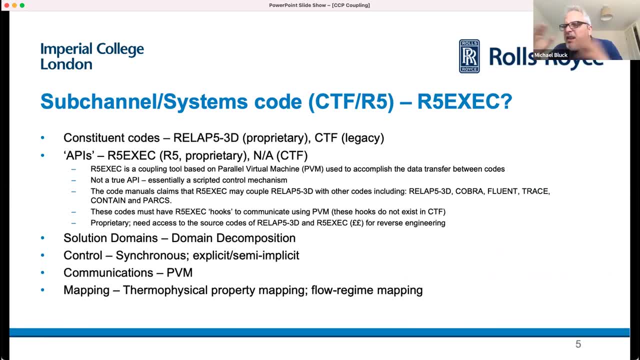 And obviously those codes are quite different in nature. So what I'm first, what I'm going to move on to, is really a sort of very top down, Top level view of some of the things we've done, And this is really a very brief and I can't say, an enormous amount. 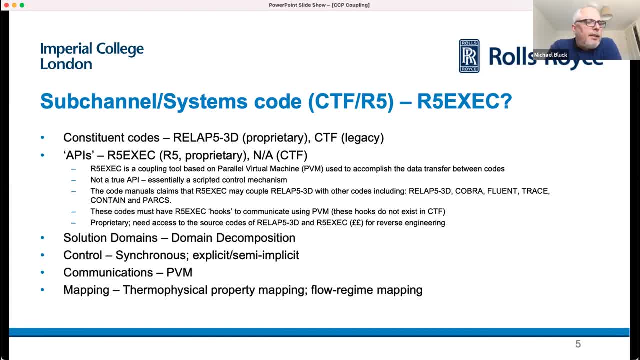 Because it's quite proprietary of what we've done with Rolls-Royce. And then there's sort of a desire to couple, in this case, sub-channel code with a systems code, In particular CTF as a sub-channel code and Relact-5 as the systems code. 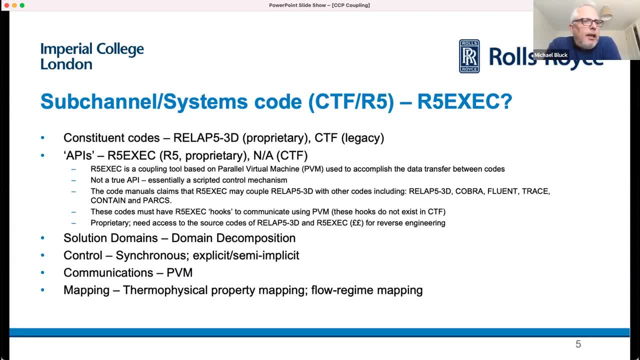 And you know, the coupling of Relact-5 in particular has been a long standing sort of aspect of its development And in particular it's embodied in terms of coupling using- well, they call it an API, It's not really called R5 exec. 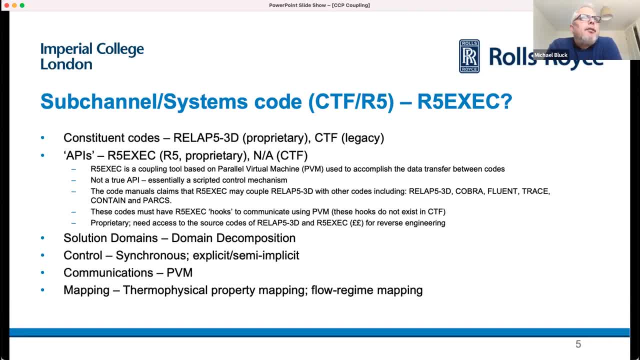 And so in this context, this was an ambition to sort of initially, you know, couple these proprietary code like Relact-5 3D with CTF, very much a legacy code, But accepted as far as Rolls-Royce and the regulator was concerned. 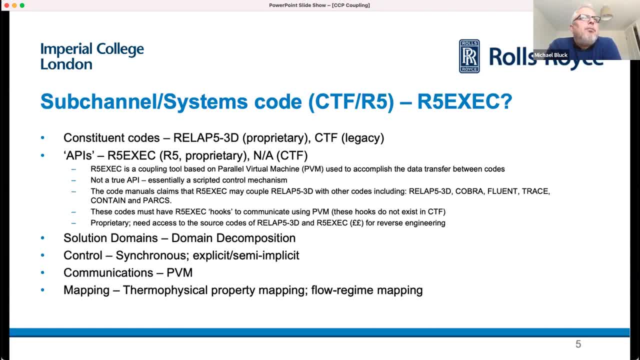 And the API that Relact-5 3D principle uses for coupling is R5 exec. Again, it's proprietary. It's a coupling tool based on PVM or variants of Used to accomplish data transfer between the codes. It's not a true API. 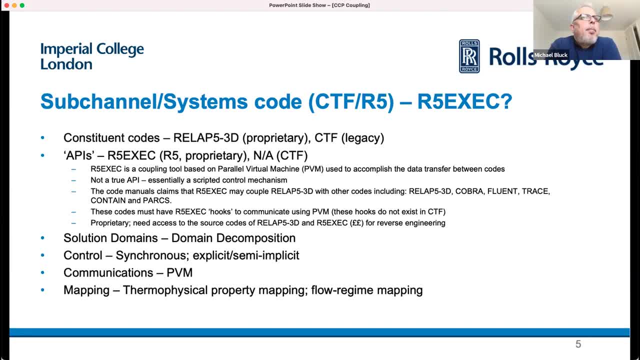 It's essentially really a scripted control mechanism And whilst the code manuals will tell you that it can couple with anything- And there's a number of codes there- The requirement here is that these codes have the relevant R5 exec hooks in them to communicate using PVM. 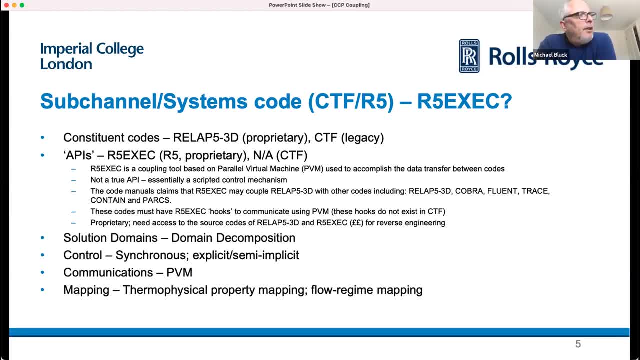 Notably, these hooks don't exist in CTF, which is a great choice to make. you could say It's proprietary. The manuals don't tell you what to do or tell you anything about the internals, Just tell you how to script it. 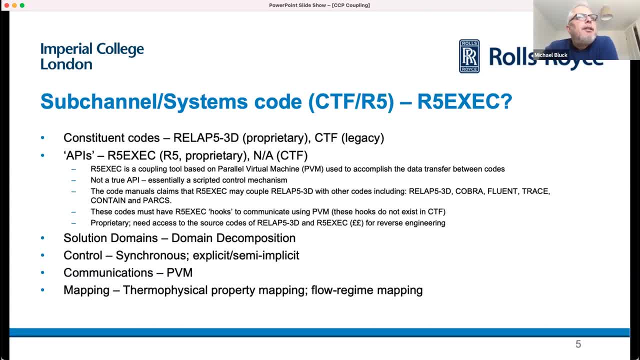 You could reverse engineer much of the stuff, but that's very expensive, Not least because of the license costs, of access to source codes And so on. It's a domain decomposition method. It's synchronous, Supports both explicit and semi-implicit communications with PVM. 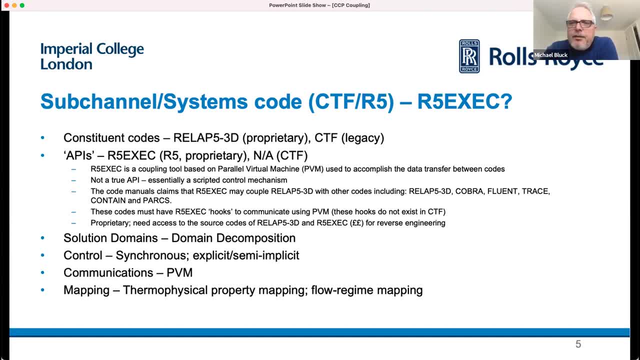 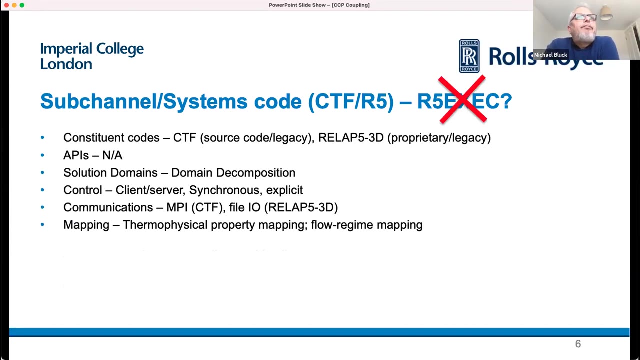 And it maps the thermophysical properties from one to the other and also maps the flow regime between the two. So this was the issues with R5 exec. It pushed us to go down a different route, Really forgetting about the R5 exec API. 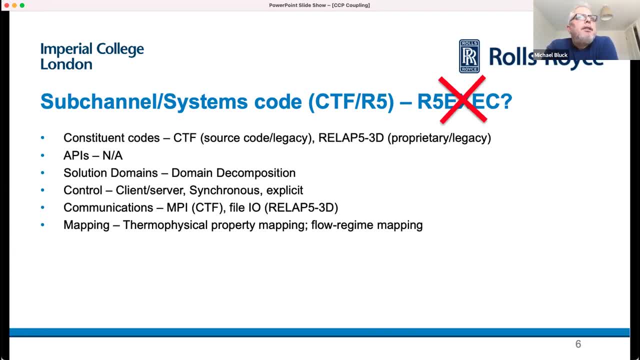 But still following a domain decomposition route with a client-server model and synchronous but explicit. And the communications: it may seem a bit clunky but we have access to CTF source codes. We can enable communications with MPI into CTF. With Relap 5 3D we actually implemented just a simple file, IO and restart mechanism. 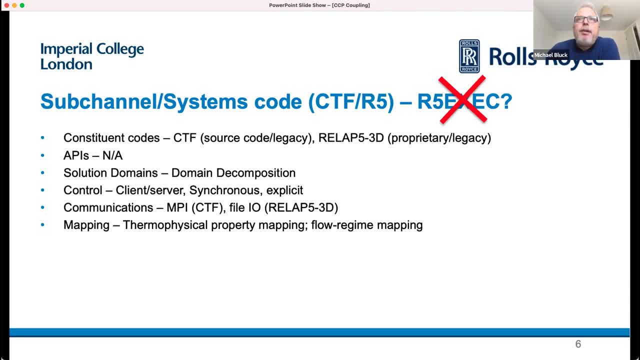 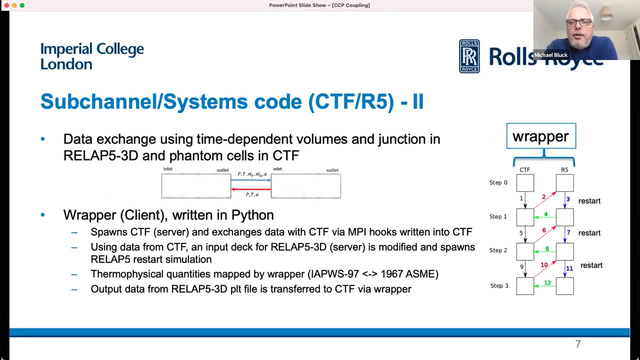 But again supporting those mappings, the same mappings. So this was quite a sort of clunky thing, Just really driven by the selection of the funders Requirements. So this sort of alternative was involved: data exchange between time-dependent volumes and junctions in Relap 5, 3D and phantom cells in CTF. 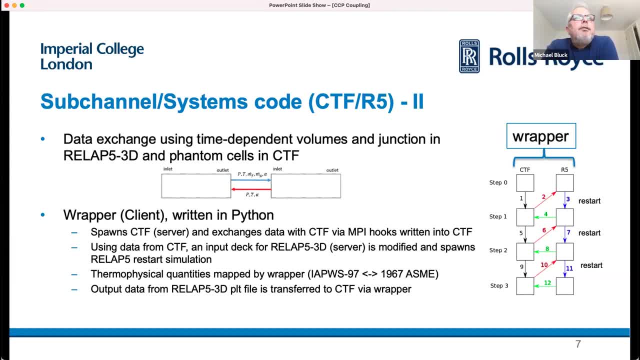 And depending on the sort of flow direction we're passing: pressure temperature, mass flow rates of both phases, void fraction one way and pressure temperature the other. And it was a client-server model, So it had a wrapper client written in Python. 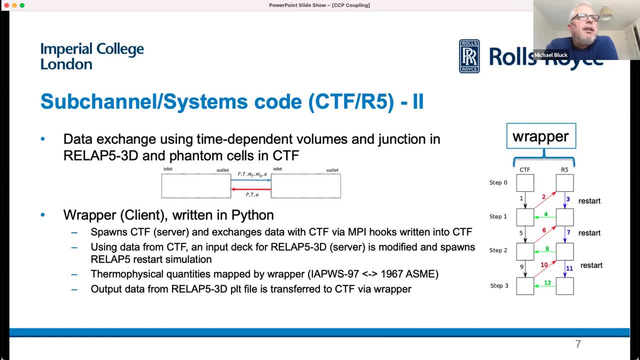 And, as you see on the right, it spawns the wrapper, spawns a CTF server And exchanges data with CTF by MPI hooks written into CTF And using that data from CTF We create, we adapt the input DEC to Relap 5, 3D and spawn a restart. 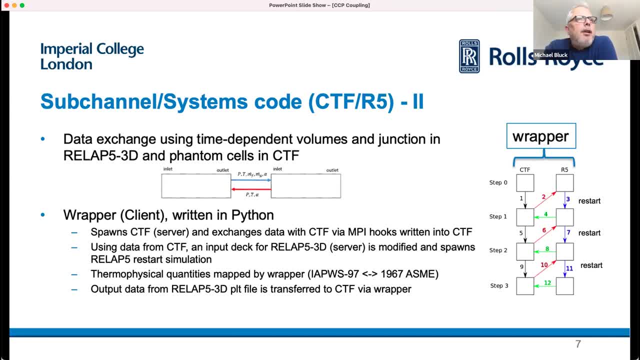 Sounds a bit clunky, But it does work. There's a need to map the thermophysical quantities Because they have different steam tables and thermophysical tables, So that's done by the wrapper And the output data. Each step is written to a PLT file. 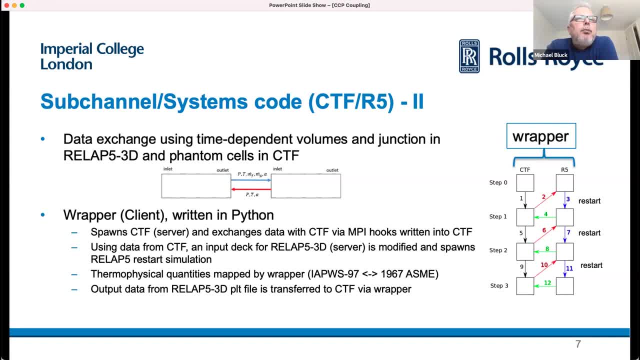 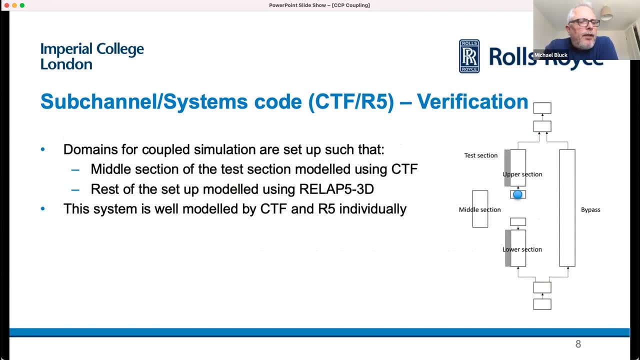 Which is transferred by the wrapper to CTF. So this is a workaround very much Not as you would possibly want to do it. So validation verification is important. So this is a verification And it's a very simple case Of a test section and a bypass channel. 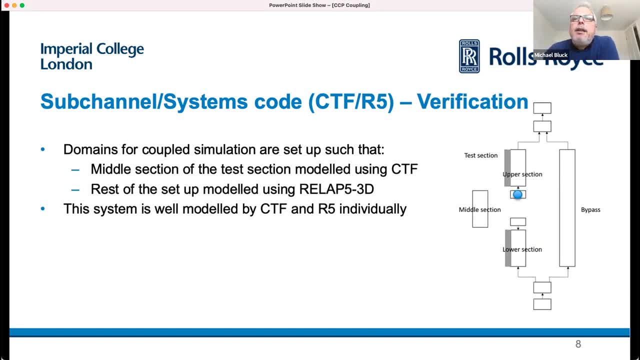 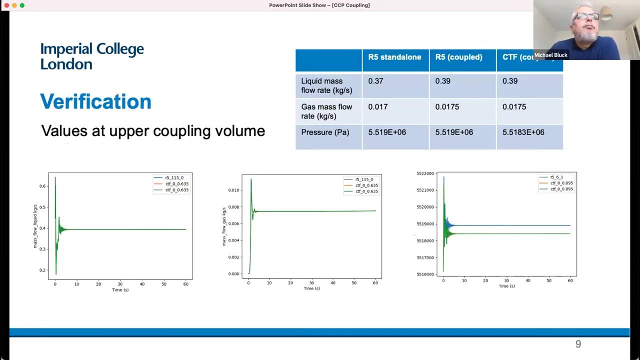 And in this case, the middle section here is modeled using CTF And the rest of it is modeled using Relap, And this is very much a verification process rather than validation, As this system overall is pretty well modeled by CTF and Relap 5.. 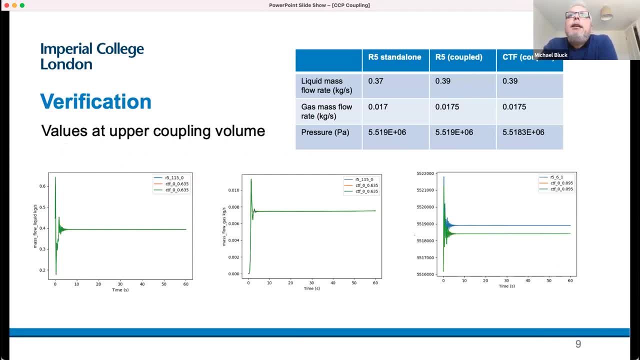 And the verification process is pretty viable. The liquid and gas mass flow rates are very well predicted, As you can see. So the possibly one issue is a sort of deviation there. for the pressure, I think, as everyone said, the pressure converges a bit more slowly. 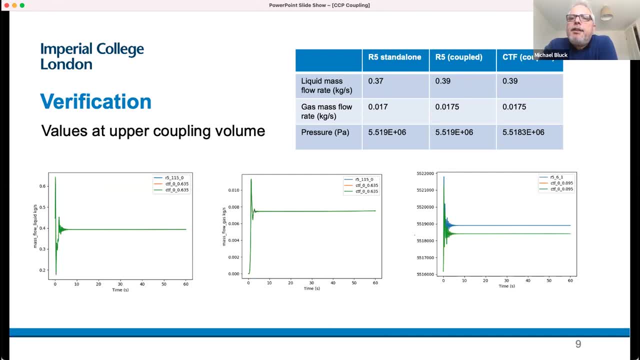 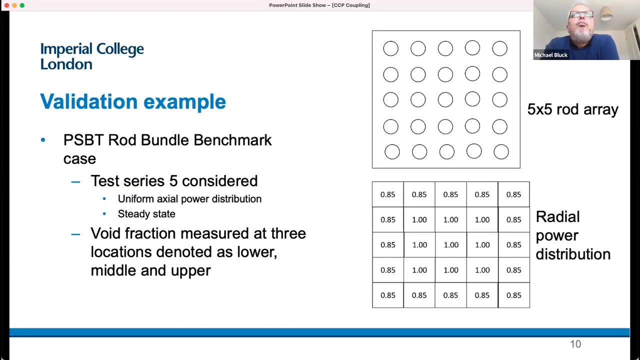 But those are small differences And this is just a verification activity To make sure that things are doing what they should. I won't be able to give any sort of more detailed and more useful verification validation Just due to commercial issues. A validation example which is a PSBT rod bundle benchmark case: 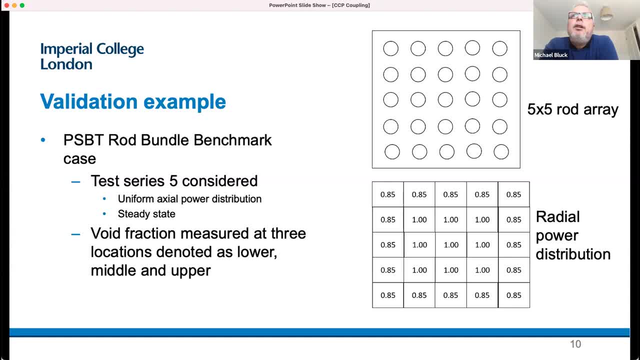 Test series, five of those considered. It's a bundle, Five by five, rod array, Uniform axle pair distribution And we're looking at the steady state And the void fraction is measured At various locations And it's got a sort of slightly inemogenous radial power distribution. 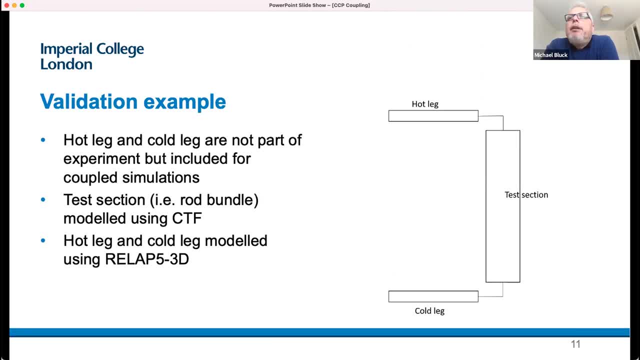 In that And all we're doing really is modeling the test section in CTF And the cold leg and the hot leg In using Relap 3D And the results. I'll go through this quickly, I don't want to go over time. 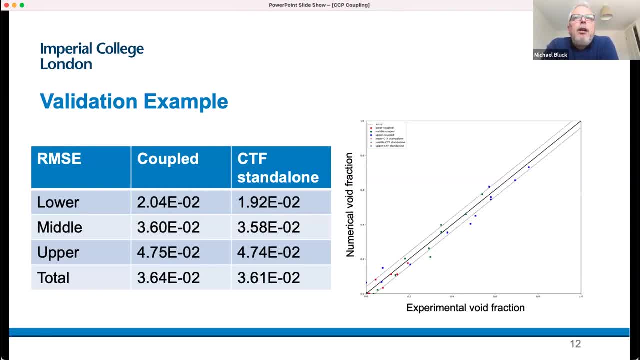 And the results again Are pleasing. You can see on the graph on the right The experimental void fraction on the on the X-axis and the numerical void fraction on the Y-axis. And there are some outliers, The the. the dotted lines indicate a standard deviation. 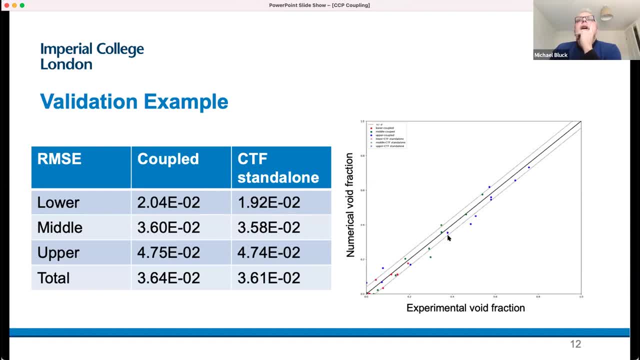 Plus or minus. Sorry the variance And and and generally the the sorts are Plausible and So Good agreement with either CTF standalone or indeed not shown on there, Five standalone. So so, in terms of 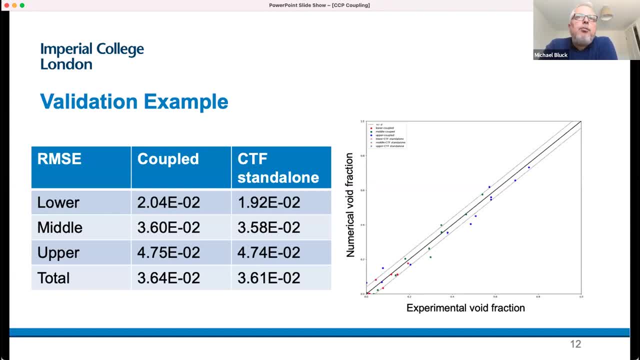 Possibly more verification and validation At all. Things seem to be working well. As I say, there are issues with the pressure And we need to look further into that. So that's, that's an example, really, of coupling In a in a sort of 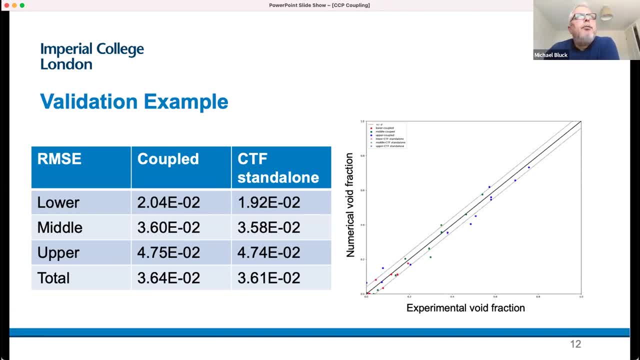 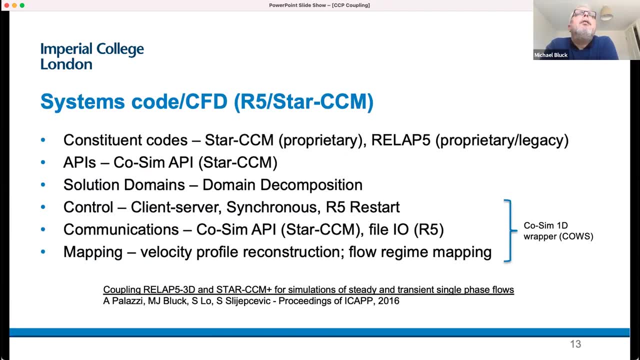 Fairly clunky way. So There It's. it's a, it's a kind of, It's a way of looking at Sub-channel code with a with a systems code. The next one I'll move on to is: 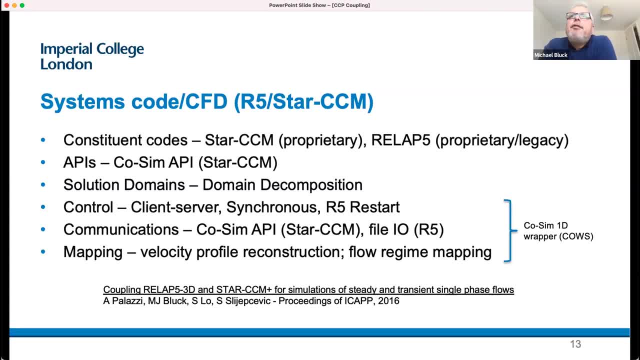 Is coupling Five with a with a CFD code, in this case star CCM. So the constituent code to a style which was the proprietary Five, again proprietary Legacy as well. The APIs: API used here Is the walls at that time. 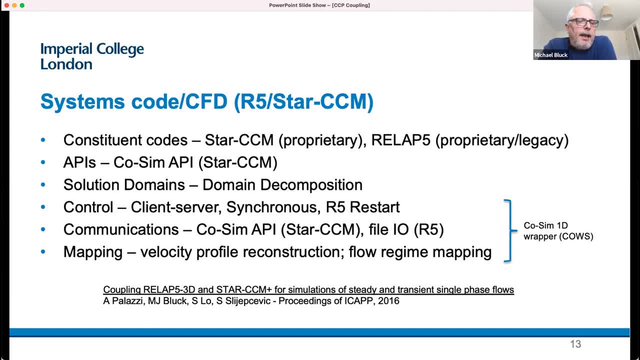 in star CCM. And again domain decomposition and it involved a client server model, synchronous communications And again, rather like the last case, due to the same reasons, broadly we react. five was was on the coupling side, was done by a file, IO and under under restart. 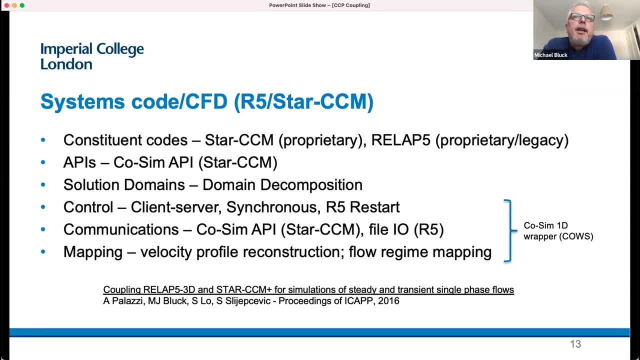 So Congo, through the K tornado, api on the star CCM side and file I on that five side And there was a essentially a wrapper acting as the client cows cosine one D wrapper, And again the mapping was was his, is is important for the coupling of CFD. you've got to go in. 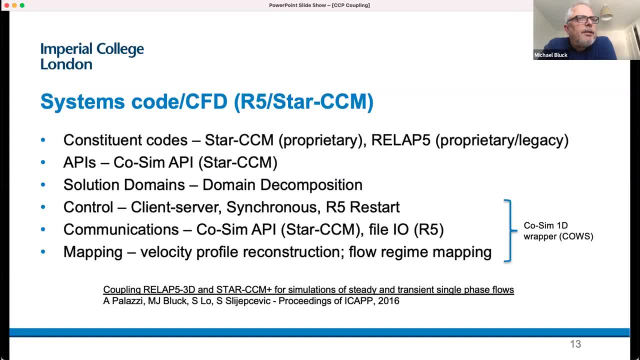 from the CFD to the systems code is relatively straightforward. Going in the other direction, you need to recreate velocity profile. You also, going back from CFD into Relap5, need to make sure that you are consistent in producing the appropriate flow regime map. 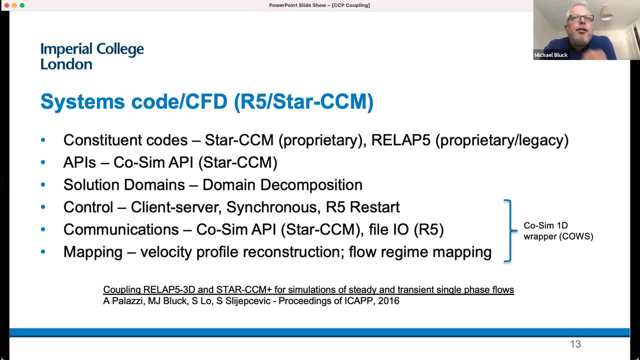 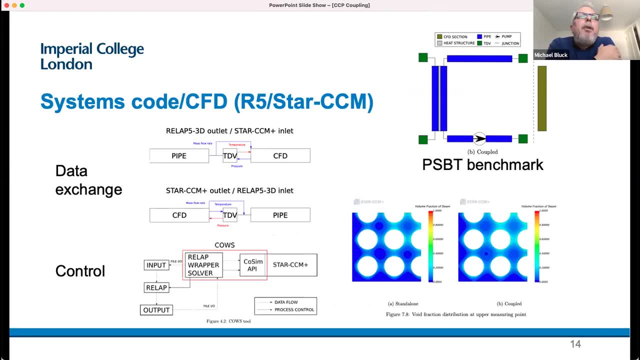 It's not just a matter of passing those variables. So as an example, here again a similar PSBT benchmark, the case you can see right. And so the blue is modeled in Relap and the green, the test section, is modeled here with star CCM. 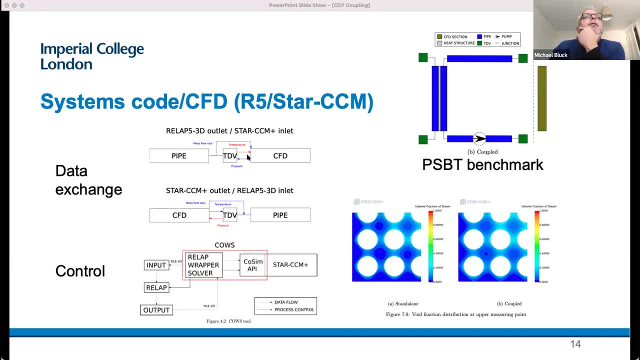 Data exchange depends on directionally dependent the data exchange passing: mass flow rate, temperatures, pressures and so on. Just for clarity, I've just put the single phase transmissions there and the control is as you see. here there's a wrapper essentially around that acts as a client. 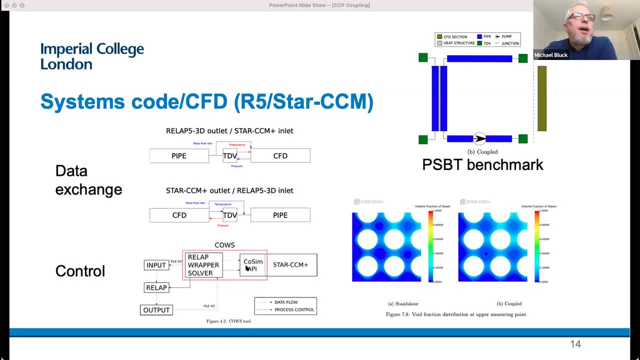 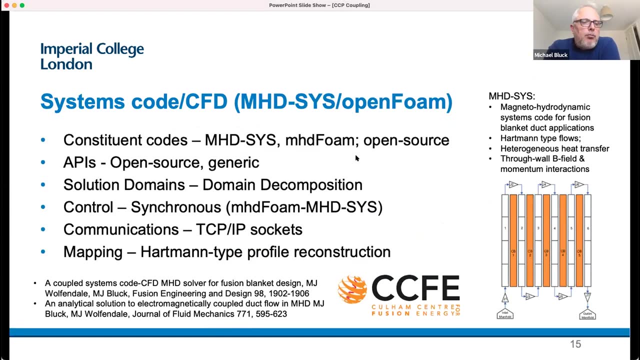 to enable and manage the communication and all those things and the mappings from one to the other. okay, so, so that was the. that was a real at five star CCM coupling, I'm sorry, um, a different case now, which was the coupling of a systems code, again in HD. 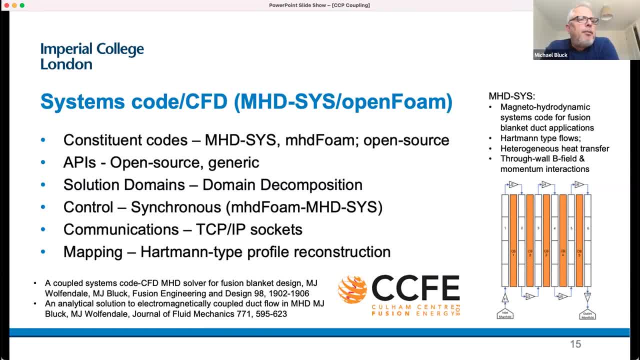 sis. so this is a magneto hydrodynamic systems code with open foam, and the advantage here is that in both cases these were open source and in-house written in terms of MHD sis. our HD sis is a magneto hydrodynamic systems code for fusion blanket duct flow applications. it, it, it deals and 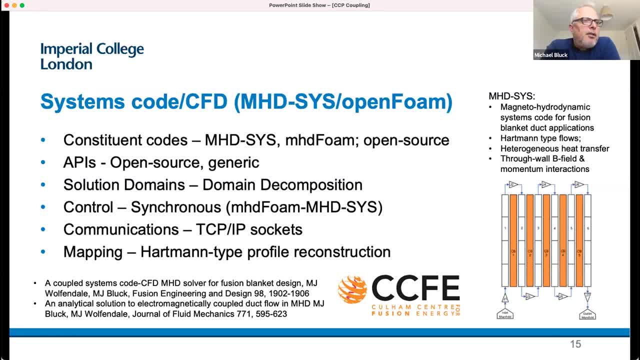 with Hartman type flows, whether it's Shercliffe and Hunt type flows. so the velocity profiles in for for when the magnetic fields are high, are very different. those in in normal sort of hydrodynamic cases, uh, including sort of wall jets and and and and so on. so so the the particular profile. 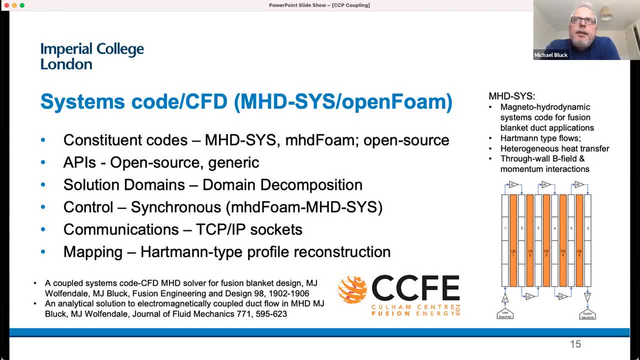 reconstruction is very different. um MHD sis also deals with quite heterogeneous heat transfer. you've got, because of the very different flows, you've got very different local nusselt numbers on on different walls of duct depending on the orientation of magnetic field, and you you've 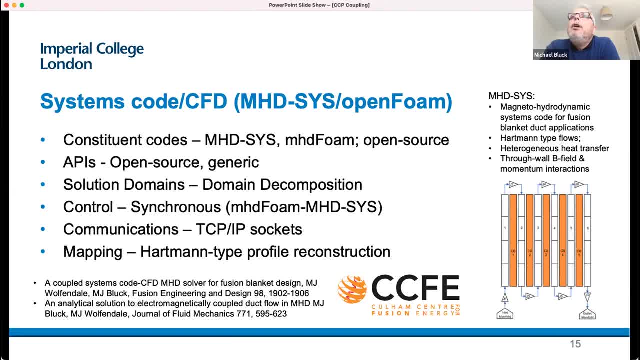 also got the potential for through wall magnetic field and momentum interactions. so the the flow in one duct actually affects the flow in the neighboring duct. okay, and so these are, these are these sort of uh. in various sort of prototype um fusion blanket applications we have flows sort of uh as a as. 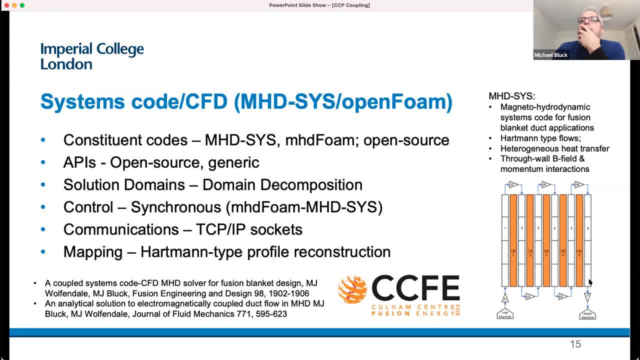 a sort of serpentine arrangement, and in order to get there in particular, you often need quite complex manifold arrangements. so whilst the systems code can quite successfully described the flows in the sort of ducts, the flows within the manifolds are vastly more complicated. so 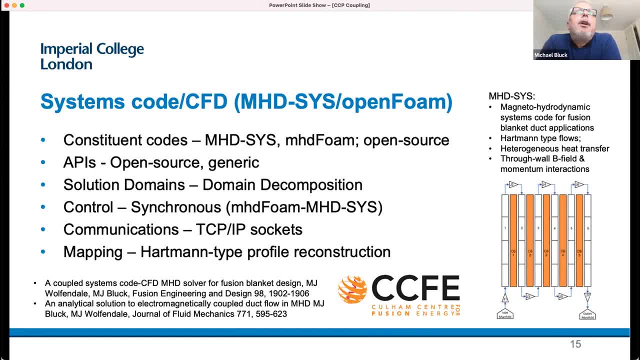 the the motivation for coupling the systems code to a cfd code, in this case mhd foam. so these are both open source and and hence quite generic apis. it's again a domain decomposition approach, that's, synchronous communications, and in this case there's not a lot of data being sent. so this 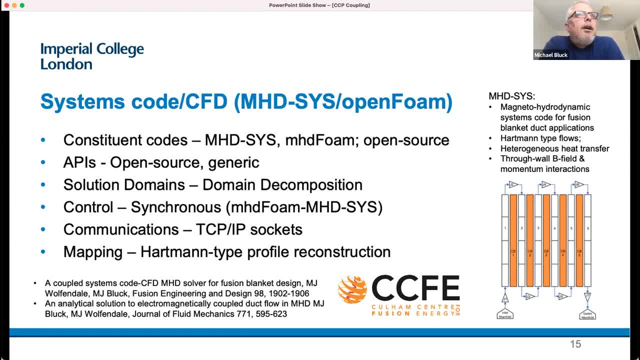 we, we just use tcpop sockets. um, one of the difficulties is most of the significant message passing interface methods. uh are there to pass quite significant amounts of data. uh sort of high bandwidth, but not so not necessarily great latency. uh, we're not passing lots of information. 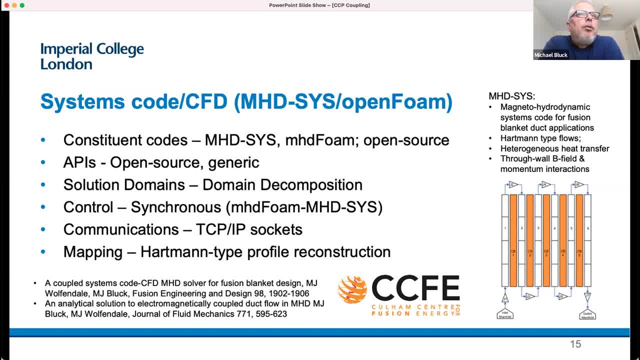 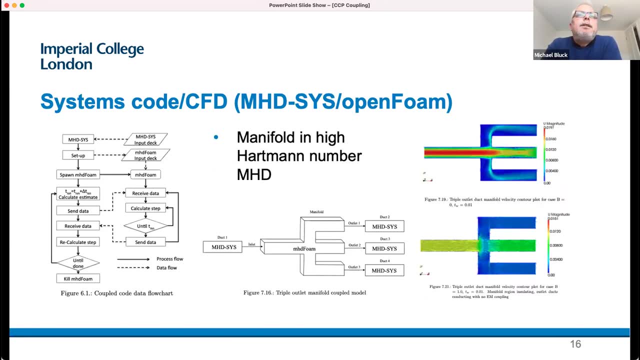 so. so it's, you know, the opportunity to see what, what just going right down to the libraries would would do. and, as i've said, the, the mapping is a good deal more complex for profile reconstruction. and this is, this is essentially the- on the left, the, the. 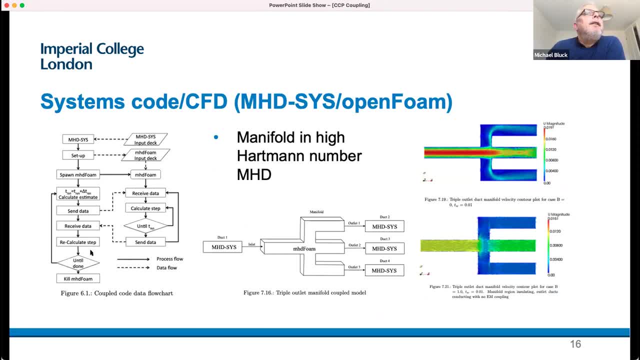 left of the left picture, if you like, is the mhd sys and this is the synchronous communications between that and mhd phone and this is controlled by a a. so this is a case where where we have a manifold so split from uh, one channel, one duct, into three. 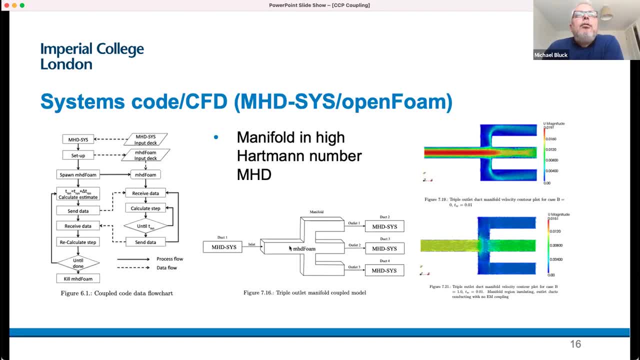 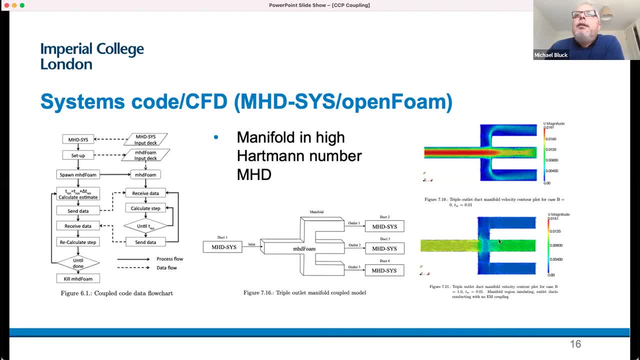 model using mhd foam. on the right you can see that the effect that changing. so so, if you like, before this on entry, the inlet and outlets- beyond what you can see on those pictures, are modeled using mhd sys and so we're modeling the, the sort of behavior of of the manifold using uh mhd foam. 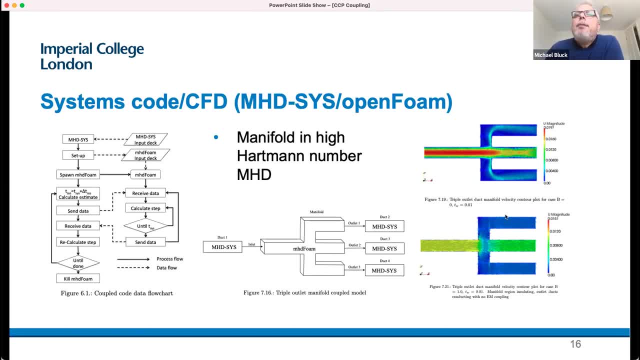 and we'll see the effect that changing the magnetic. so this is no magnetic field in the. in this lower case we've got a very significant magnetic field and it radically changes the flow, as one might expect. okay, so that's really just an application where we have sort of full control. 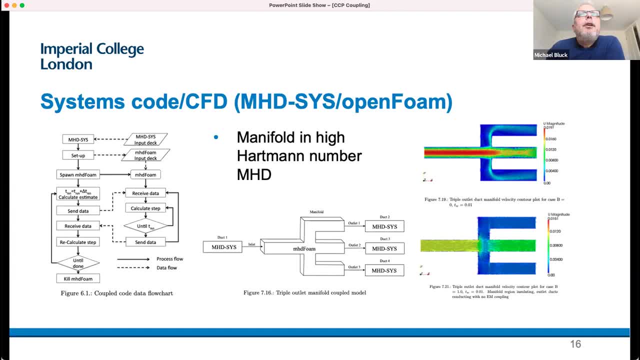 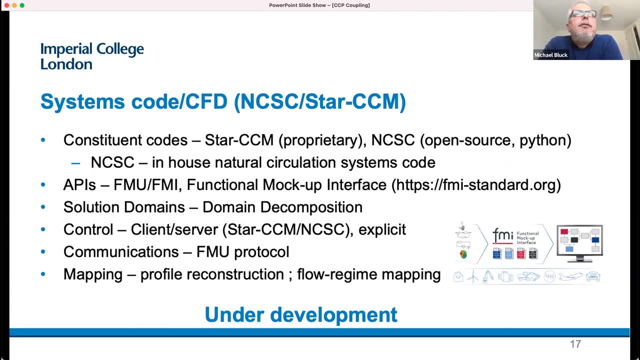 if you like, and full access to, to codes, um and just one sort of final one again. this is looking at a sort of again the development of, of interfaces and so on and various protocols. we're we're looking at coupling, involvement or developing the coupling between star ccm- again again proprietary um- with an in-house. 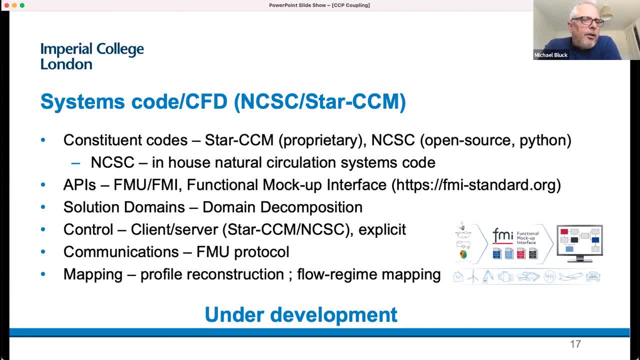 or open source. uh, natural circulation system of code. it's a, it's a test bed for dealing with situations that most systems codes don't deal very well with, surprisingly, which is is sort of low flow rate natural circulation design between star, ccm and in house. so that's, that's really really good. 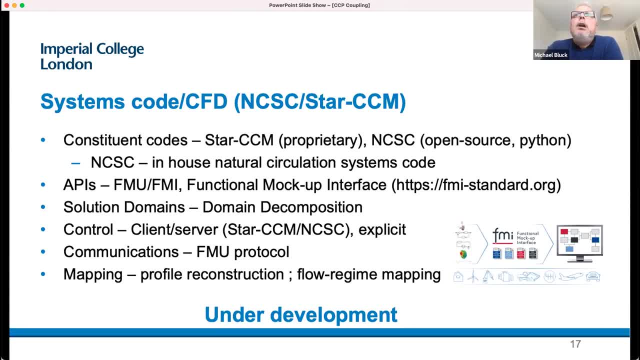 natural circulation um and and so. again, that's written in-house. what we're particularly interested in is deploying the functional mock-up interface, api, that's that star ccm. relatively recently um incorporated um the fmu, fmi, and there's a link there to it um so it's 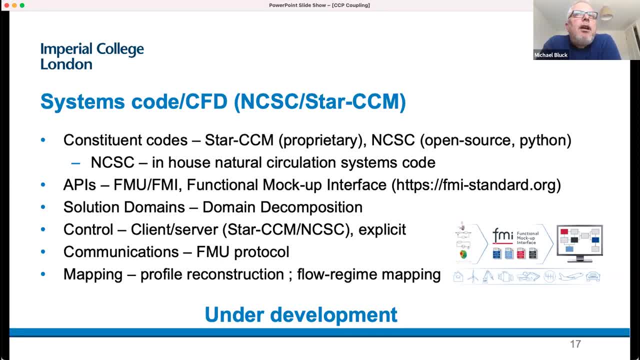 open source. again, a domain decomposition. it's a client server model, again explicit, with star being the client um and the communications are all managed through the fmu protocol. again, we'll look at profile reconstruction, flow regime mapping. uh, much of so this is still under development. uh, really, a lot, of a lot of what our sort of work has been is is looking at how we practically 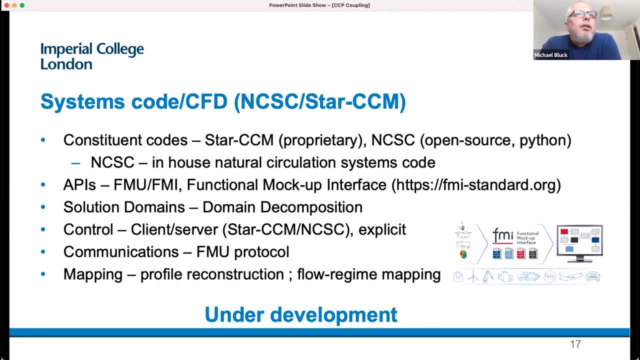 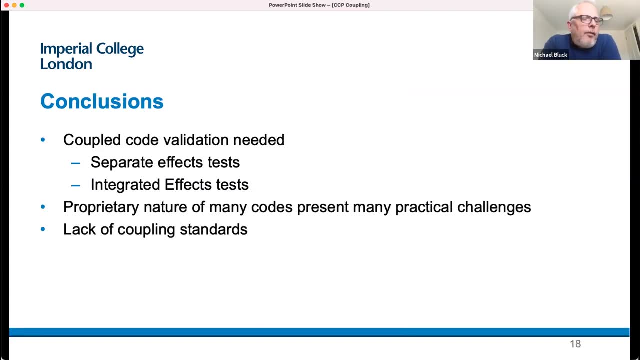 implement in a broad range. so with, with, with the, with the release of fmu, uh, in star, that's what we're intending to, to sort of evaluate really as much as anything. so that's still under development. so just to, just to, i've just tried a very broad overview of some practical elements really of and a few cases of. 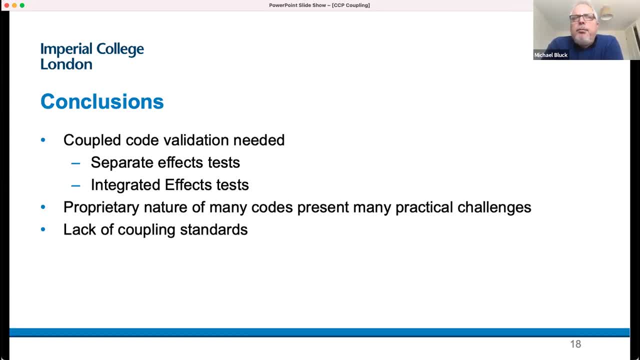 um outlining sort of the implementation and what what affects certain um choices make. um, as i've said, been said before, uh, you don't get around things doesn't get you that far just because you've coupled two accepted codes. you still need to do all the separate and integrated effects tests. the proprietary nature of many codes present. 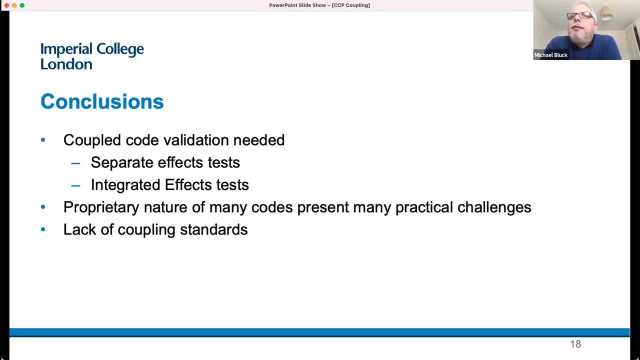 present many practical challenges. so there's a, there's very much, perhaps a dissociation between what can be done, so computation scientifically, and the and what what in practice? uh, um, you know, developers need to do and there is clearly lots of, there's lots of coupling but um paradigms and protocols, but there there's a lack of a standardization, um, 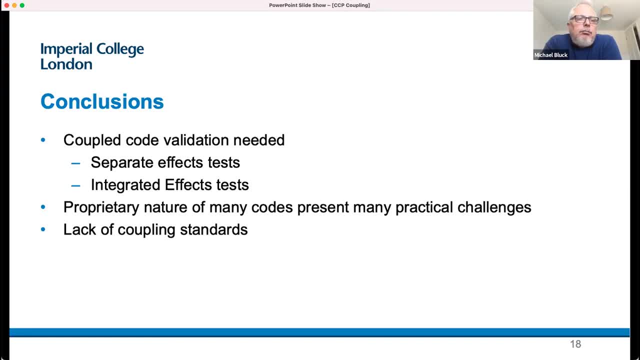 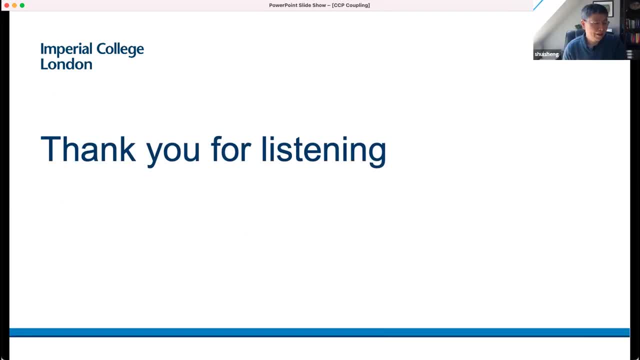 i'll end. i think the whole thing will come to a close, um, almost on time. okay, thanks, uh, mike. uh, a lot of information there and it's really interesting. and now can we just have a couple of questions for mike and then, um, hopefully, we probably will just uh move to general discussion. 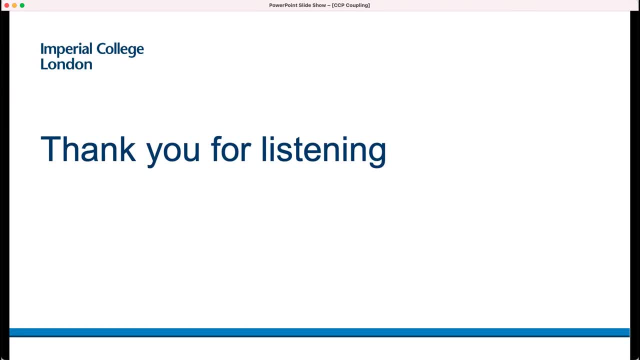 uh, my name is vincatz. I'm from Liverpool University. My question is, you know, is there a reason why you have used STAR-CCM for coupling? Is it better than ANSYS Fluent? There's a little bit of. we have a very close relationship with STAR-CCM. 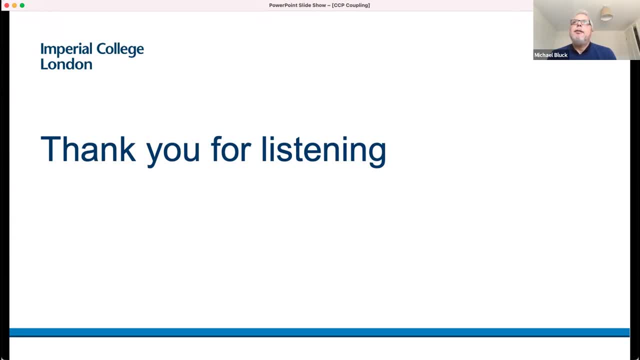 It's not surprising. It grew out of our department. So again, it's one of those things I'd reiterate and say often it's practical things like that that can influence the choice of code, And so often it can because the vendor has made a technology choice. 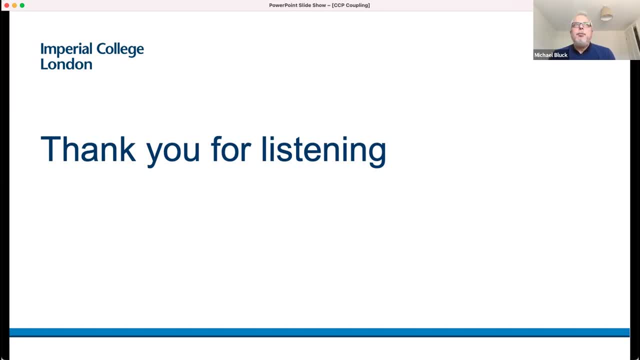 Okay, In many ways Fluent would be easier for a bunch of reasons. And one other question, if I could ask: when you couple CTF, when you couple CTF with relap, what parameters have been exchanged between those two codes? 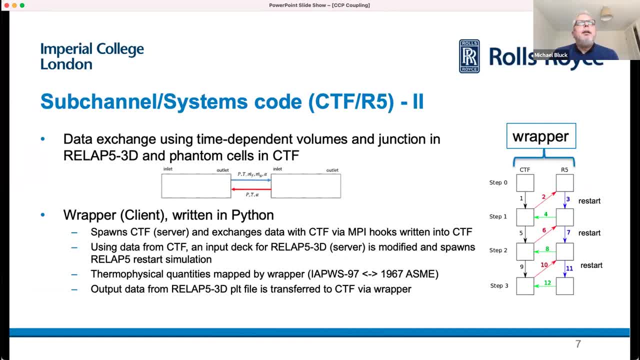 So it depends on the direction of flow. but pressure, temperature, mass flow rates and void flow. So it depends on the direction of flow, but pressure, temperature, mass flow rates and void fraction one way and pressure temperature and void fraction the other. 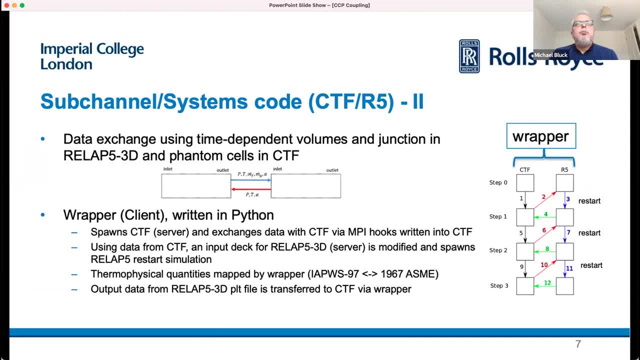 Yeah, In part that's because there's the need to map between the thermophysical quantities. They're using different steam tables, which is annoying. But yeah, so that's what we do. Thanks, Mike. No problem, Mike, just following that question. so it's nice to see that you're actually working on this to begin with.